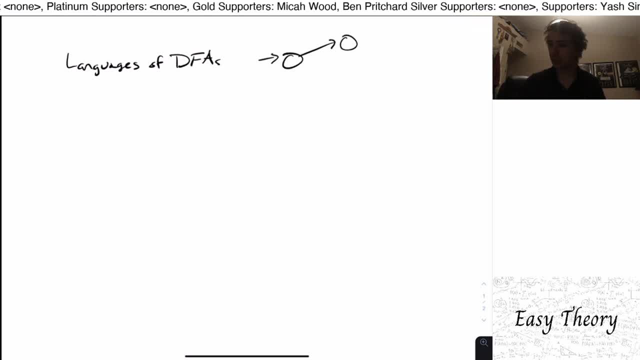 and what are those? Those are just a state-based machine that looks like this potentially has some transitions. some states are final and the language of these DFA's are just the set of all strings that are accepted by this DFA, by any DFA. So those are what we call the languages of 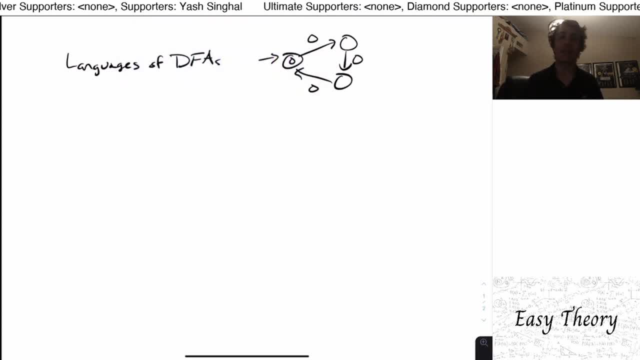 DFA's, and what we're going to be doing is we're going to give a name to these languages. So we're going to say: a language is regular. So this is actually a term that we'll be using over and over and over throughout this lecture series. So a language is regular if it is the language. 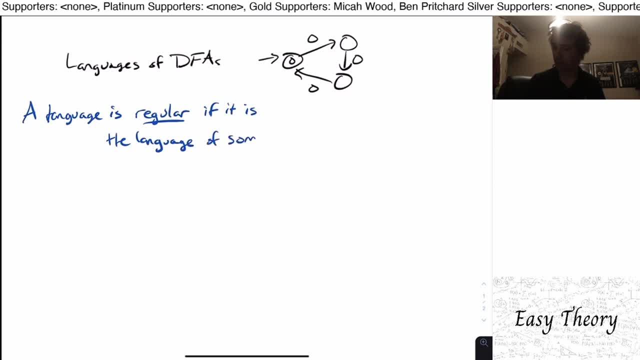 of some DFA. So as long as we know that a DFA exists for that language, therefore the language is regular, And any language that doesn't have any DFA for it cannot possibly be regular. So let's just do some examples here. So sigma star. So is that regular? 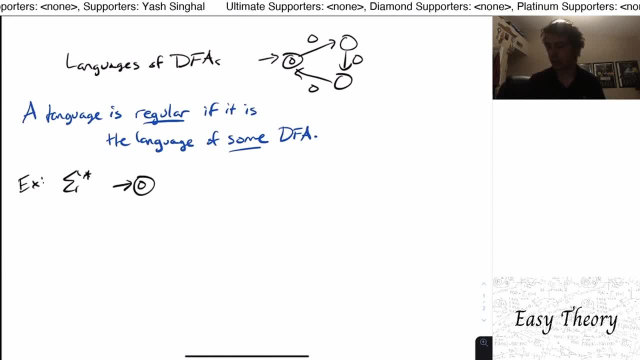 And it turns out it is obviously because we can make a DFA like this. So let's say 0, 1 if sigma is the set 0, 1, just as an example. But here we just make a single state DFA that loops. 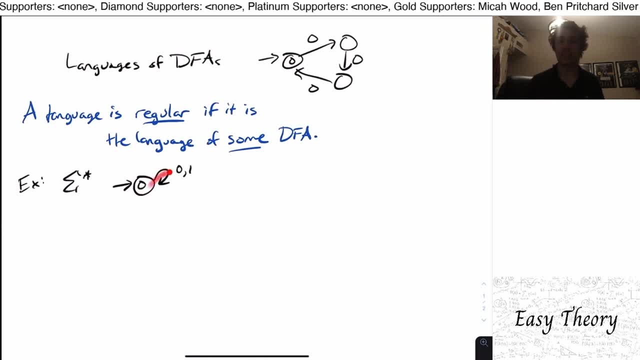 overooo, and therefore, since every string is accepted by this little DFA right here, therefore this DFA right here corresponds to this language And then therefore, that implies that this language right here is regular. So this it. so what we can say is that sigma star is regular. 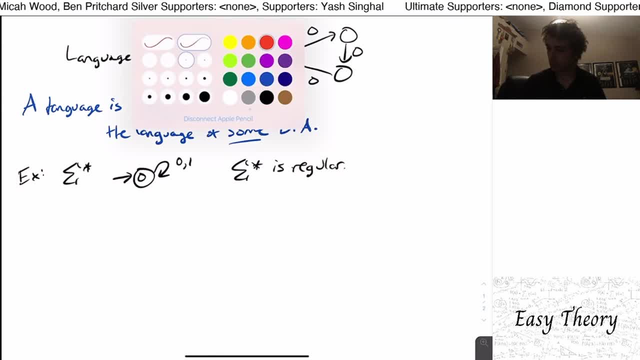 Maybe I should get rid of that. So having this DFA here implies that sigma star is regular On the opposite end of the spectrum. if we have the empty set, we can do almost the identical operation that we did with the DFA we had before, but instead we make a non-final And clearly 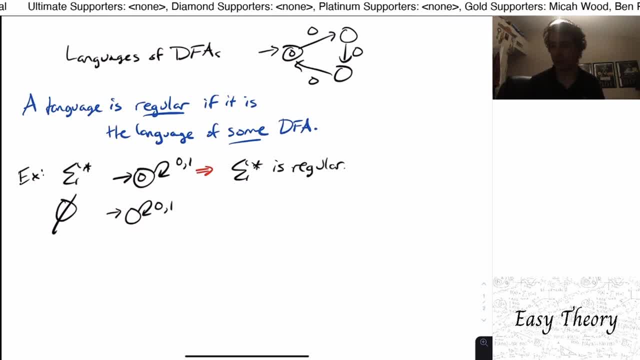 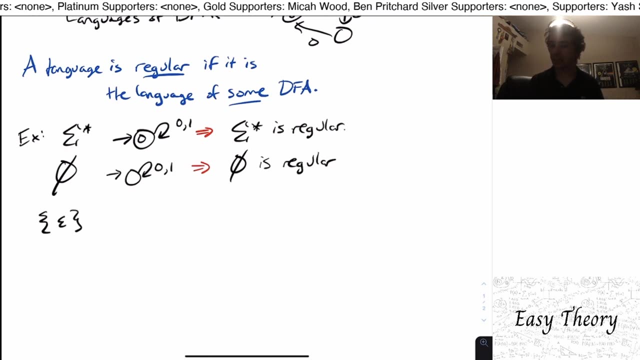 since there is no final state here. therefore, we will never accept- And this implies that the empty set is also regular. A little less trivially, we could say: have the language containing a single string be empty string, And in order to make a DFA for that we need two states. 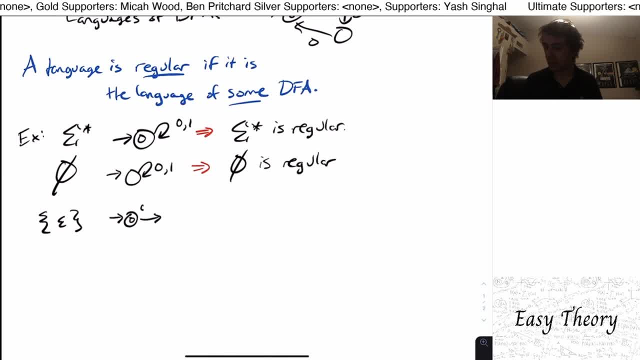 it turns out, And what we can do here is to do something like this: So instead of having one state, we have two states, And here we notice that in order to accept anything, we have to be in this state. So we can do something like this, And here we notice that, in order to accept 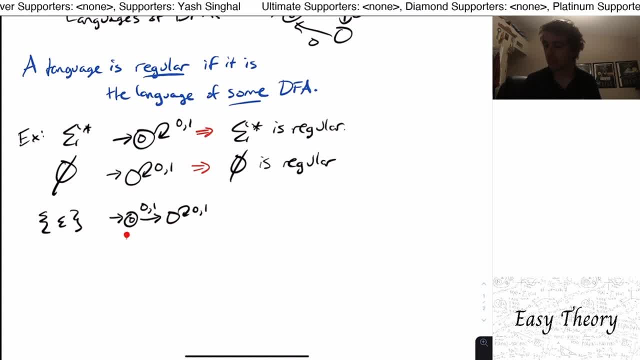 anything, we have to be in this state. And here we notice that in order to accept anything, we have to be in this state. And here we notice that in order to accept anything, we have to be start state right here, because the other state's not final And the only string that stays there. 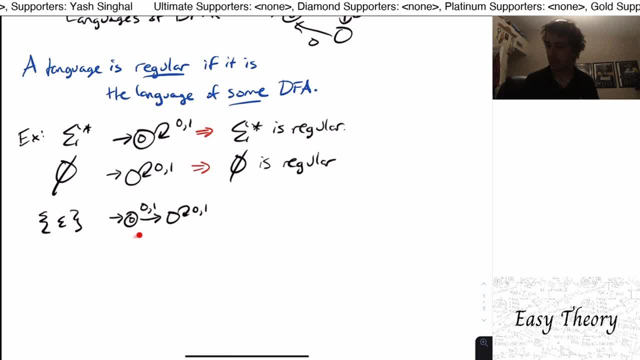 is the empty string, because if we have any string that is not empty, therefore, we end up at this other state over here. So this DFA accepts exactly one string, which is the empty string, and that's what this language is right here. So this implies that that language is regular, But notice. 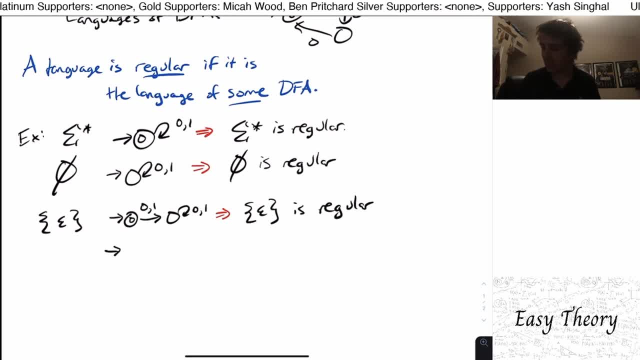 what we can do here If I take exactly the same DFA but instead I flip which states are final and not final. whatever this is, this is also a DFA And so therefore, whatever that is, it's also regular. But what this is is just taking every single string that is accepted here and making 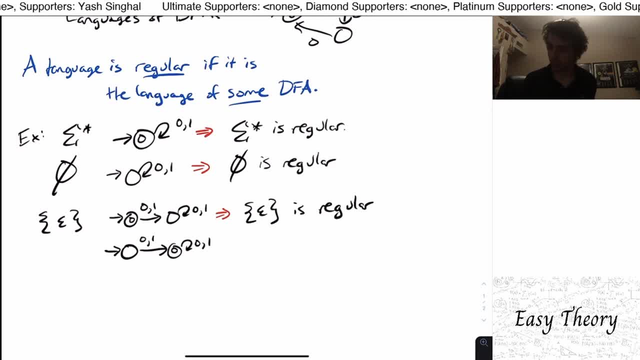 it not accept over here, and vice versa. So this language is actually a regular DFA And so what we can do here is actually equal to sigma star minus set, minus the one that we had before, aka every possible string. take away the ones in the language that we just talked about, right? 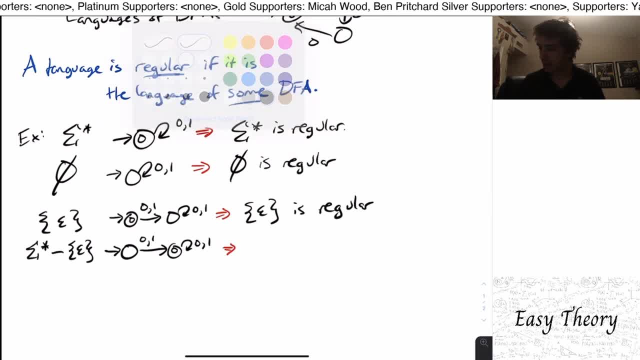 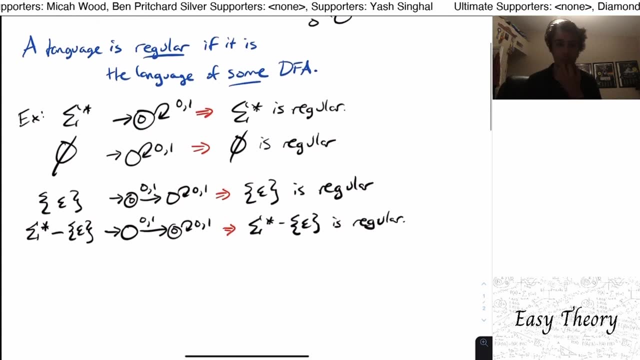 here. So this of course implies that sigma star minus the empty string is also regular. And there are many other examples that you could put. You could find, you know, you could find things that you can actually make a DFA for Cool. So these are a bunch of examples of some. 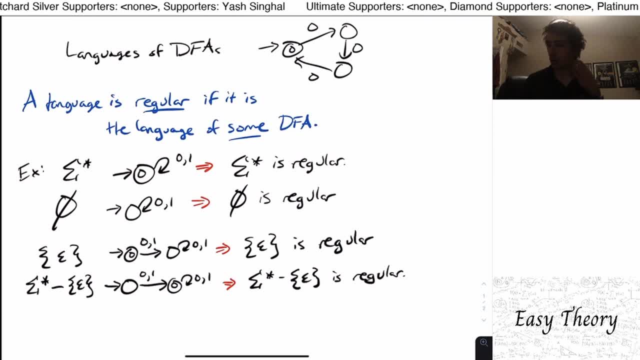 regular languages. The point here to always remember is that a language is regular, that's the name of the language. if it is the language of some DFA- And there are actually some circumstances where we do not know how to make the DFA- but we know that it actually exists And that's all that.